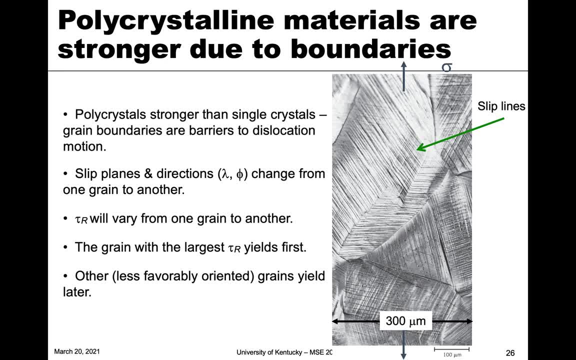 And so that causes barriers to these dislocations moving from one crystal to the next, because they, uh, in effect have to change orientation. So that contributes to a strengthening. so we can think of very loosely of these grain boundaries as barriers to dislocations moving from one plane. 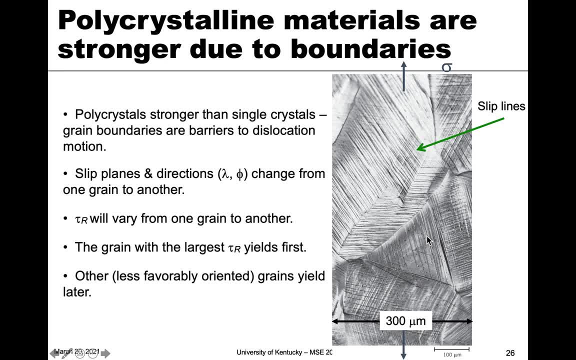 one crystal to the next. So our resolved uh, therefore the resolved shear stress that occurs from one grain to the next will be different. Um, and so what happens is the, the grain with the largest resolved shear stress, will yield first, and then others will do so later. 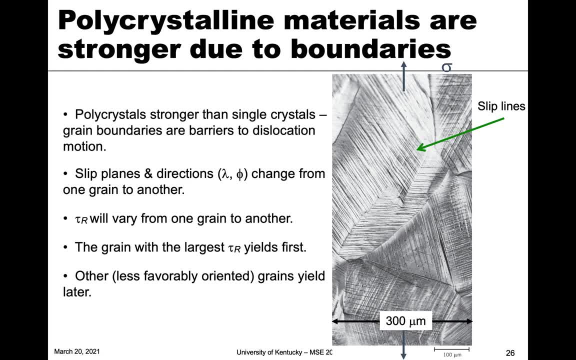 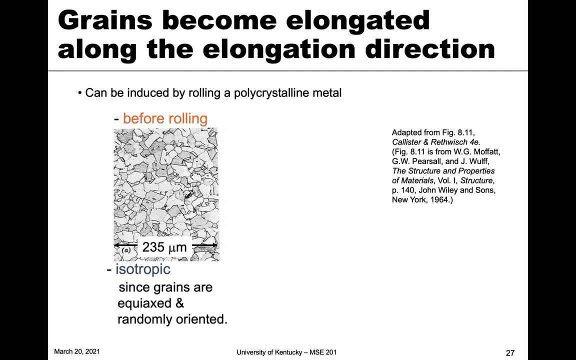 And so they provide some strengthening to this material. So we can also think about, um, uh, some different things that can happen. So let's say, we have this kind of drink grain structure here. So the grains here, they're not perfect spheres by any means. 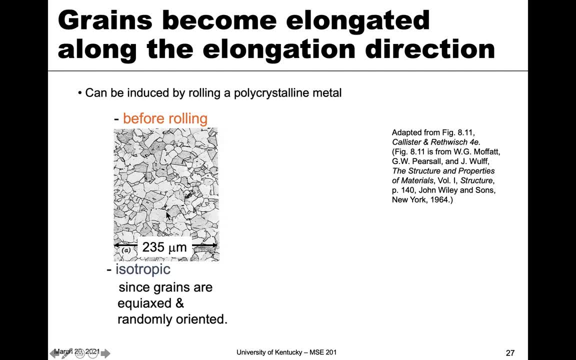 but for the most part they're uniform in direction right. There's no preferential direction. The shape is kind of um random and what we call equiaxed. So the same in all directions. So there's no preferential directions. 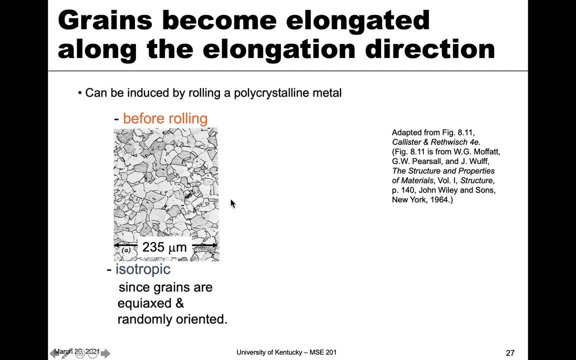 say this direction or this direction, So they're what we call equiaxed And because of this, um, this is an isotropic material, because we would expect the properties, for example, mechanical properties like yield strength, to be the same. this direction and this direction and this direction, and so forth. 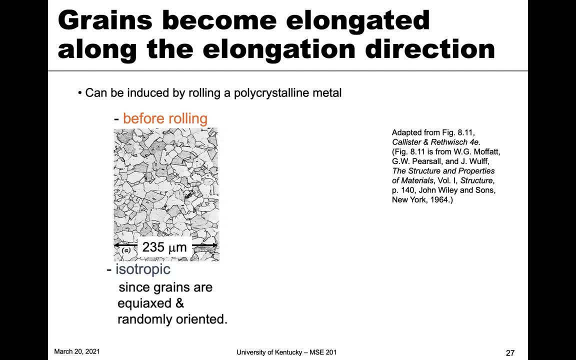 So it's isotropic, the same in all directions. So you know again. we- we mentioned this point before when we talked about polycrystals- is that they tend to be isotropic because they're, they don't change. 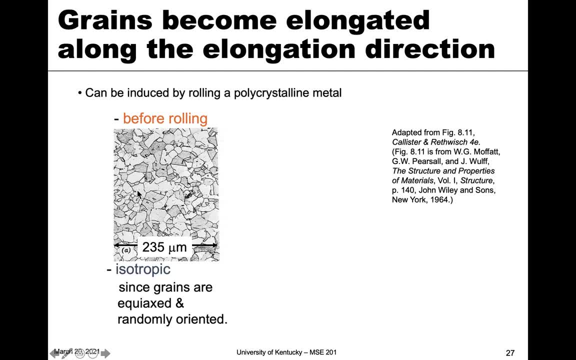 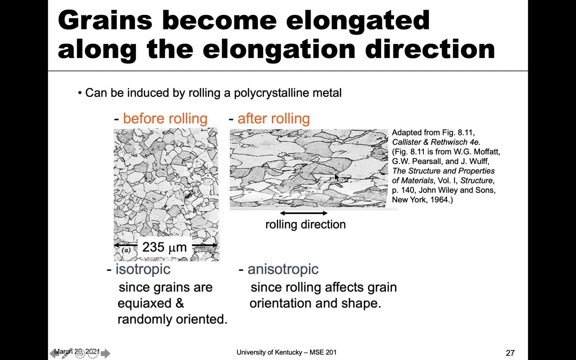 um, depending on direction, like a single crystal does. However, let's say that we roll it, So when we roll it, these grains actually become elongated along the road, What We call it the rolling direction, And so in this case, there is a preferential direction. 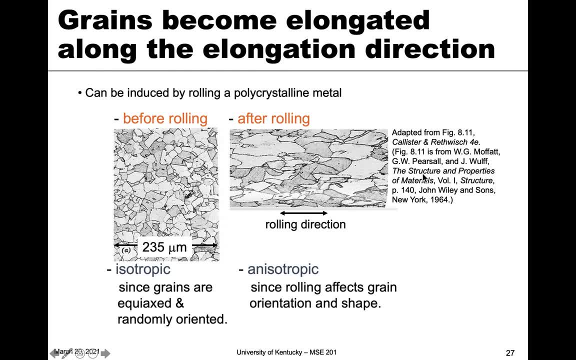 They're not. they are no longer equiaxed because they're longer in this direction and shorter in this direction, And so this is known as an anisotropic material, because we could expect that the properties in this direction versus perpendicular to it are different. 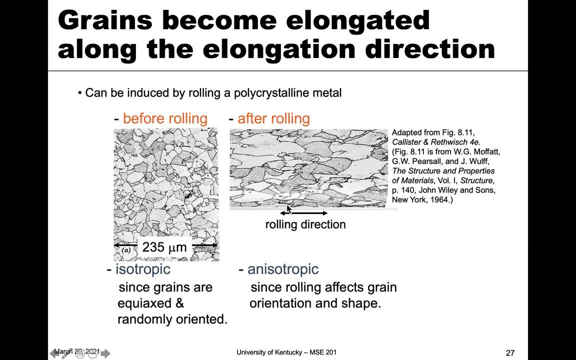 And so rolling affects the orientation of the grains, The orientation of the grains, The shape and therefore the properties, And so and again to. to deform this by rolling, we would have to plastically deform it. Um so let's look at an example of this anisotropic behavior. 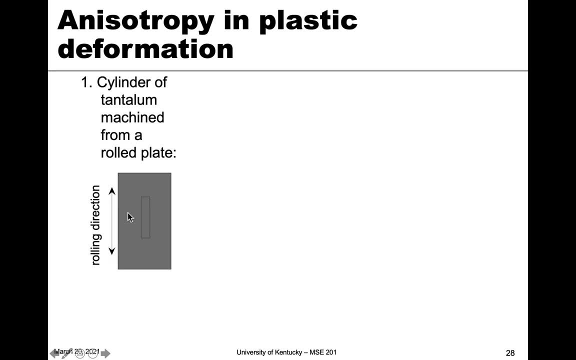 Let's say that I have a rolled uh plate of material, uh, tantalonium, not a very common material, but let's say I have that Um and let's say that I um make a cylinder from. 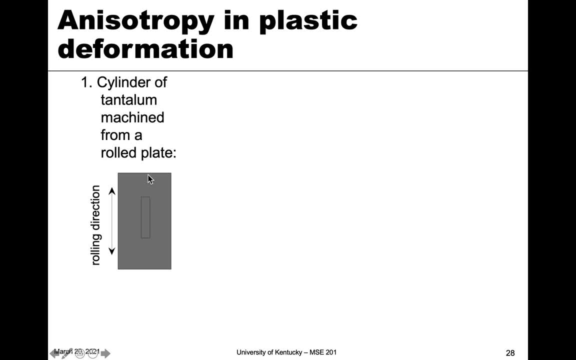 from this plate. So I cut a cylinder out of this material and it's parallel to the rolling direction. So let's say then I then fire that cylinder as a projectile at some target. So when it's fired at the target it's going to impact and therefore change shape. 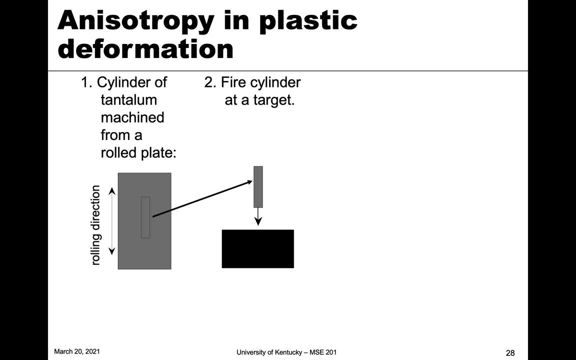 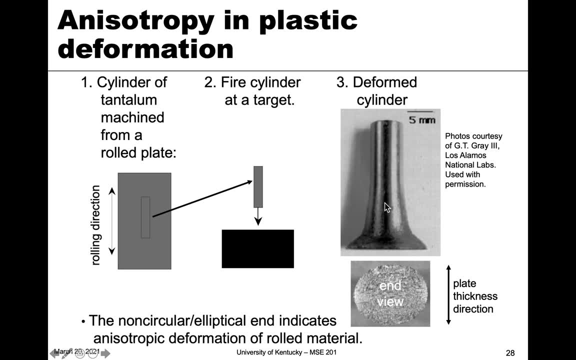 It's going to basically compress, because we're basically applying a compressive force, and so it plastically deforms, And so this is the impact portion: It's plastically deformed into the uh. when it's impacted into this flat uh, 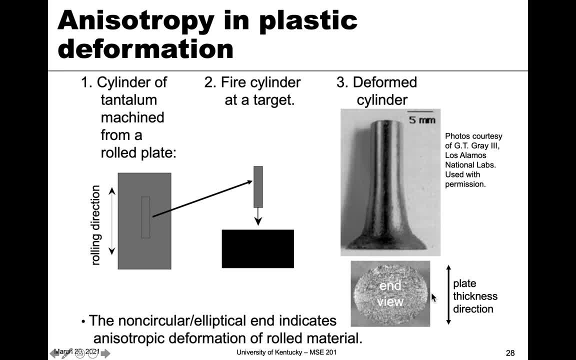 target. However, the um, the deformation is not uniform. So if we look at it from a top view, the end view, we see that actually um, this direction is the plate thickness, um direction. So essentially we're talking about the 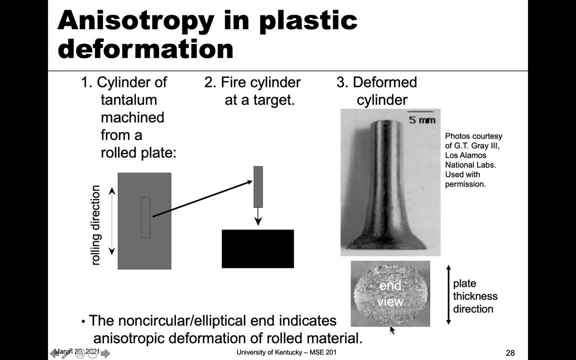 the original plate over here, And so we see that this um distance is different than this one, even though it starts out uniform, where this distance and this distance are the same, And that's because we have that um anisotropic deformation. 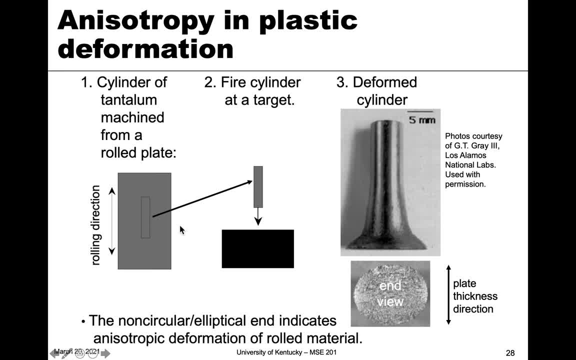 right, Because the rolling direction uh acts differently than the other directions And so we get this elliptical type or non circular type shape because of that rolling and that anisotropic deformation in this material. So that's just some of the ways that